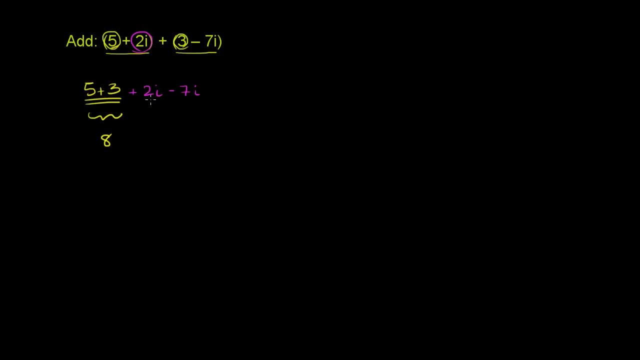 the something is the imaginary unit, the number i. If I have 2i's and I take away 7i's, then I have negative 5i's Minus 7 is negative 5.. So then I have negative 5i. So when you add these two complex numbers, 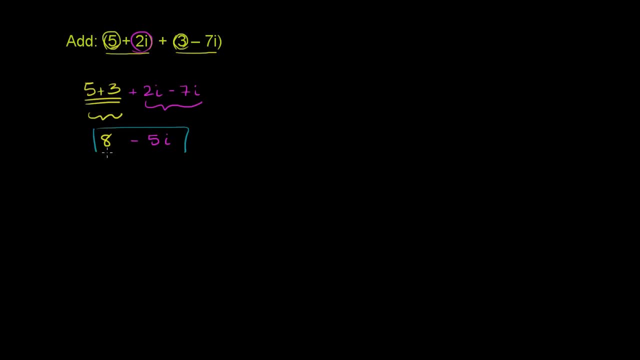 you get 8 minus 5i. You get another complex number. It has a real part and an imaginary part. 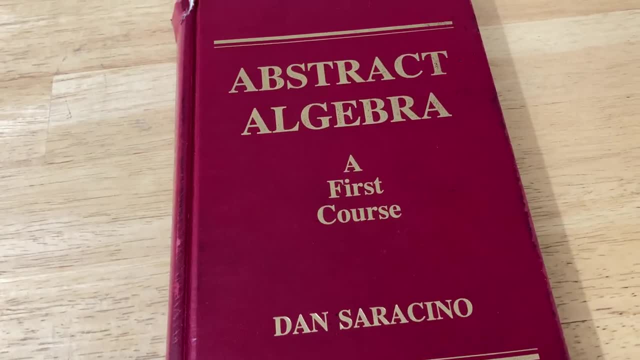 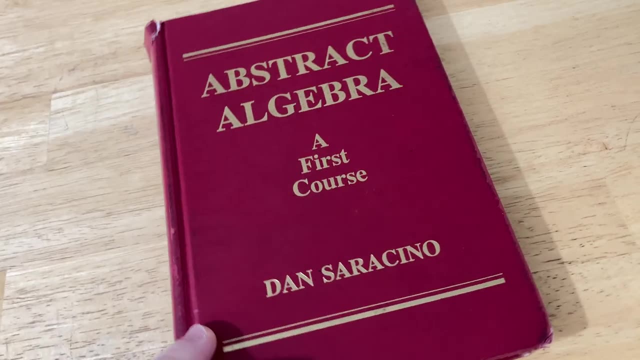 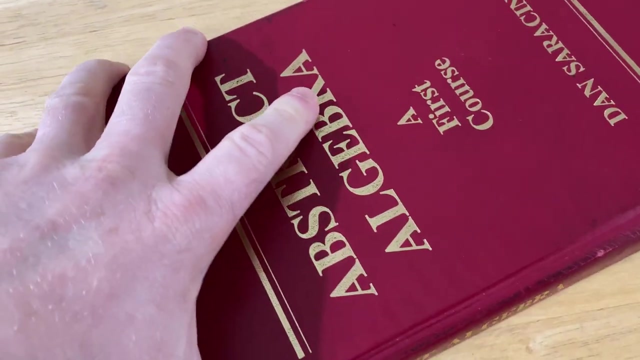 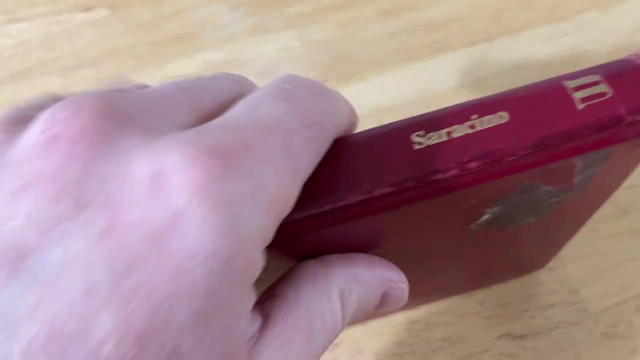 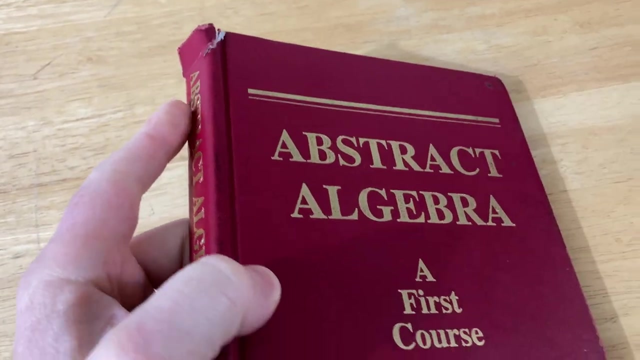 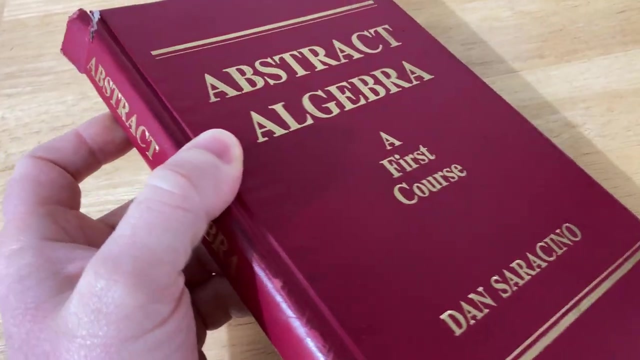 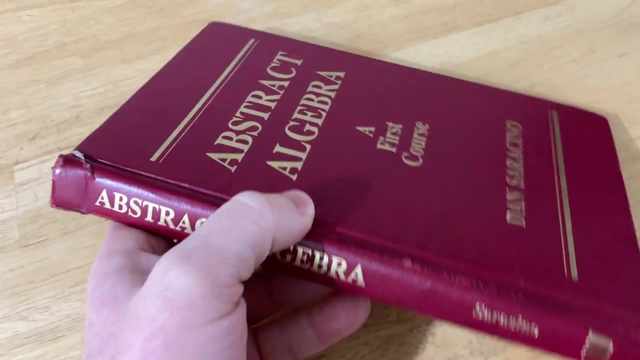 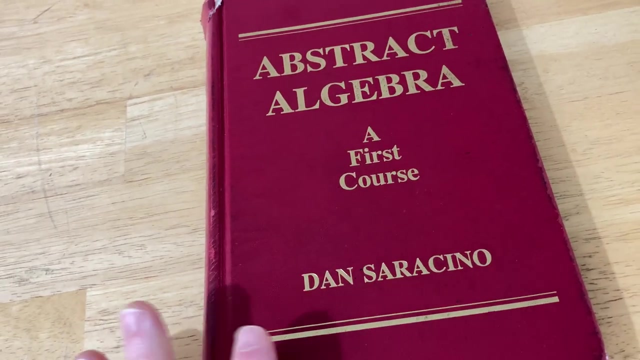 Hi, in this video I just want to show you one of my books. So this is a book I've had for a really long time, I guess about 15 years now. It's called Abstract Algebra, A First Course and it was written by Dan Cerachino. And you can see my copy here is pretty worn and this is my fault just for moving it around on the bookshelves and throwing it in boxes and rearranging things. This is what happens to books after a while. I really wish my copy was in better condition and it's entirely my fault. So I thought I would just make this video just to talk about this book and tell you whether or not you should buy it, if you shouldn't buy it, who's it for, the pros and cons. I'll leave a link in the description to this video to this book. So in my opinion, this is probably like the easiest Abstract Algebra book that you can buy. 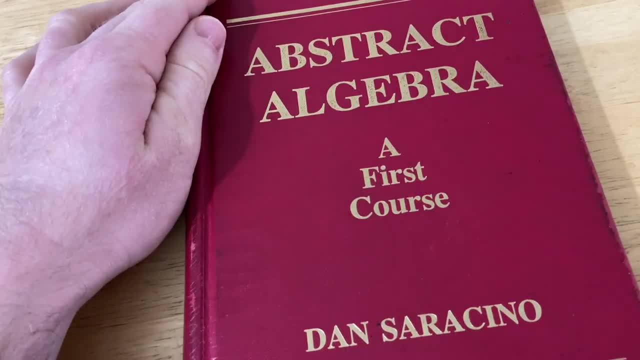 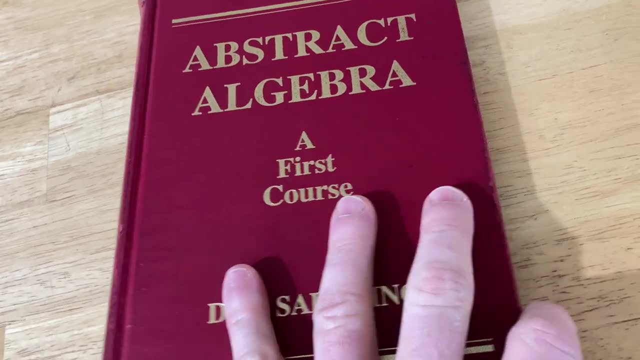 It is definitely for beginners. It is not a perfect book for various reasons and we'll talk about why. And it's also a very good book for various reasons and we'll talk about